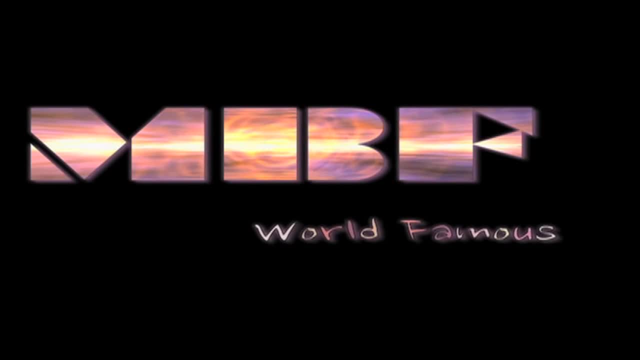 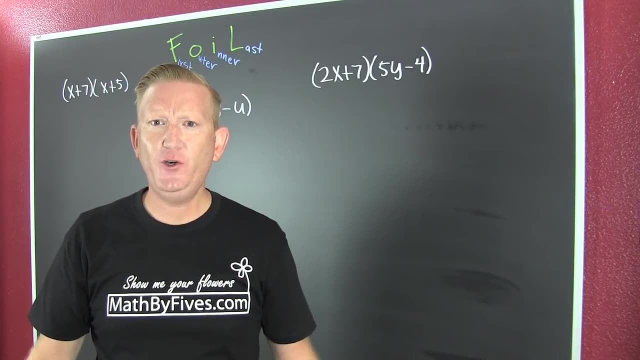 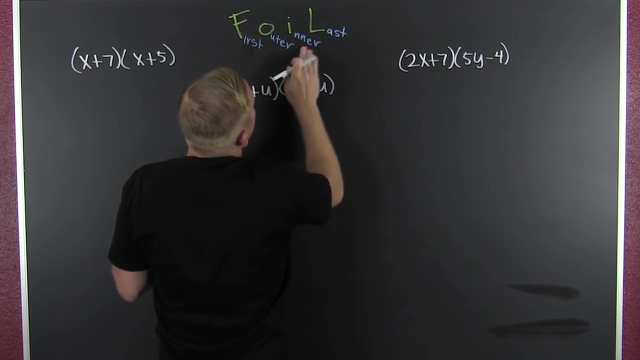 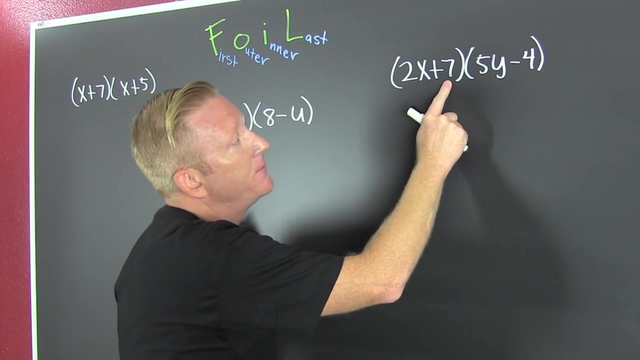 First outer inner last. Ha ha Foiled again. What are we talking about? First outer inner last? What are we talking about? Foil First outer inner last. What's it for? It's for multiplying out binomials. What am I talking about? I'm talking about two terms times two terms. But first we turn On over here. 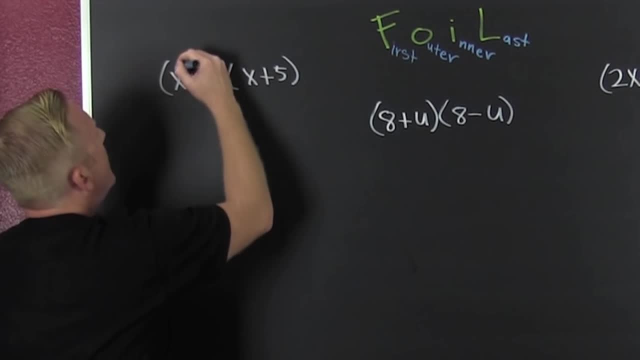 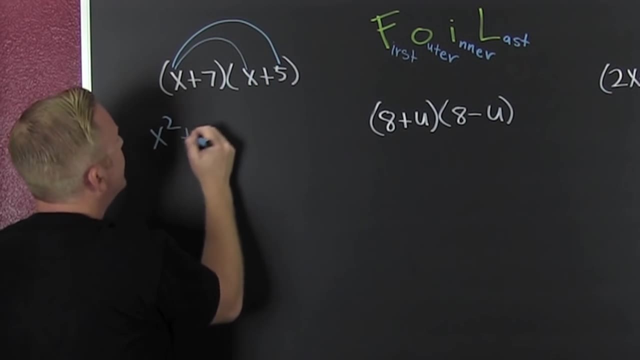 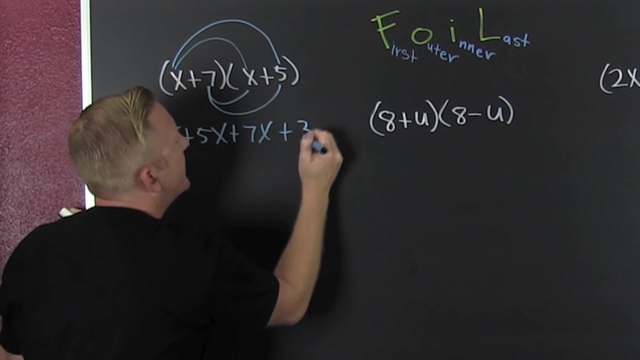 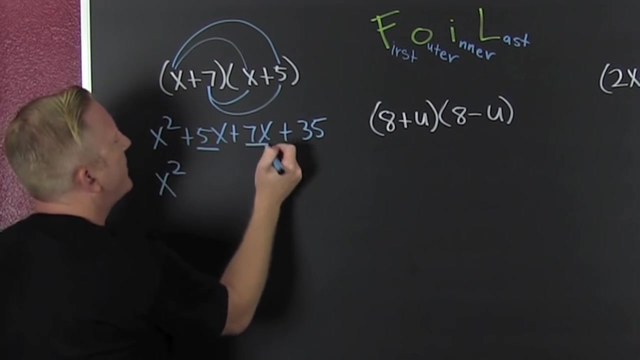 Oh boy. So then we first: That's x times x, or x squared. Then we outer: Oh boy, That's plus 5x. And then we enter: That's plus 7x. And then finally we last: That's plus 35. And then we gather, collect and combine. Gather, collect and combine. We find we have like terms. Like terms are terms with exactly the same variables raised to exactly the same powers. 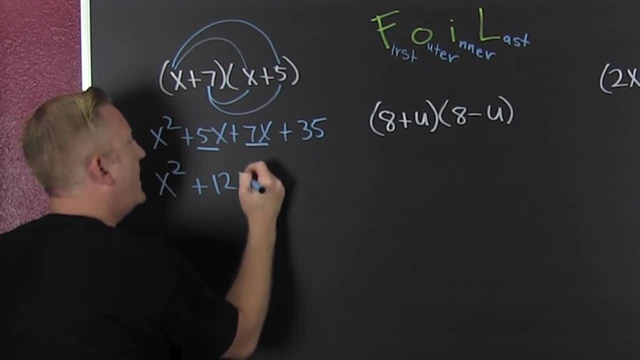 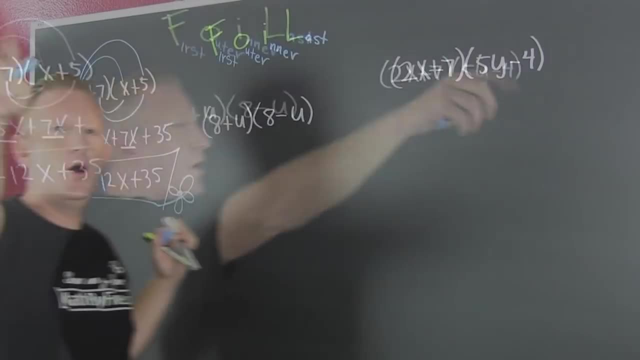 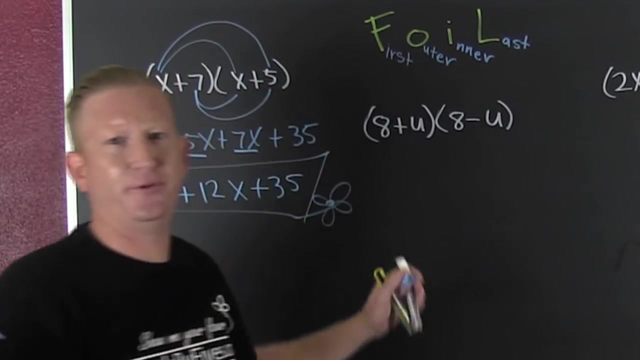 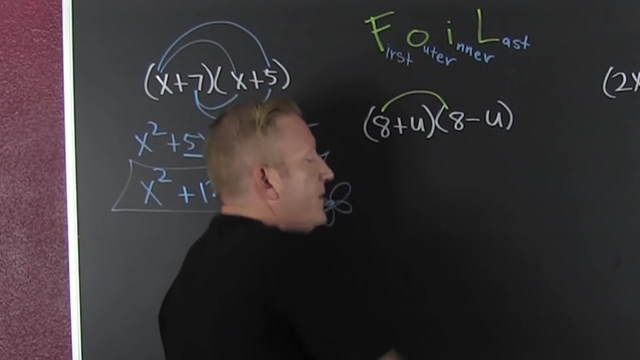 Oh yeah, baby. So then 5 and 7 is 12x plus 35.. Boxing flower. And then next, Whoa Shall we go and do the No? We'll do this intermediate. example 8u: Don't, don't, don't Foil. We first, First outer. inner last, We first That's a 64.. And then we outer. 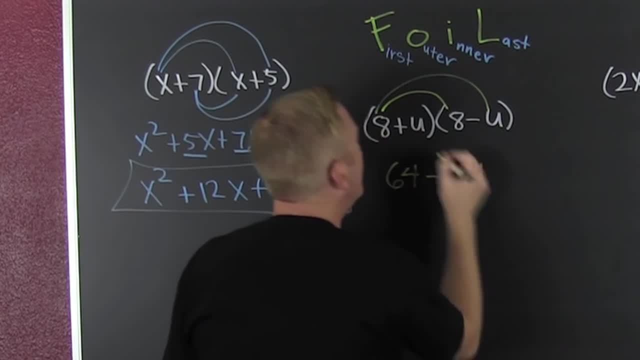 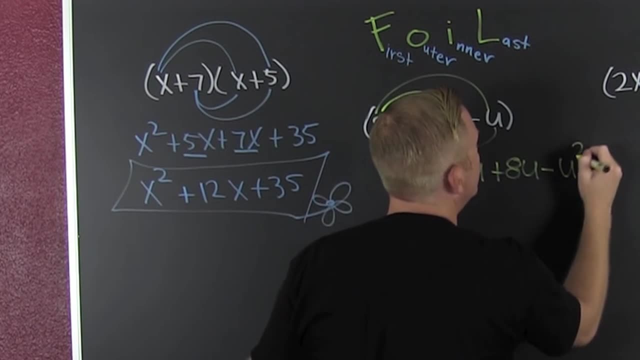 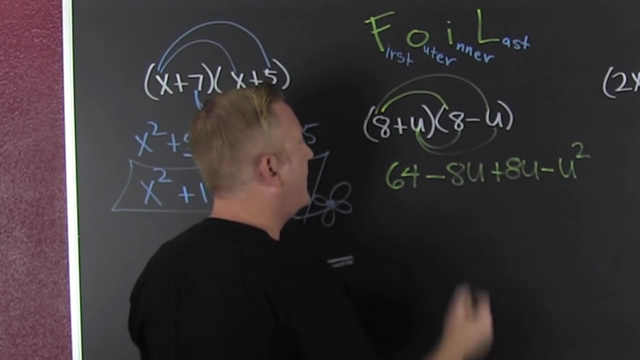 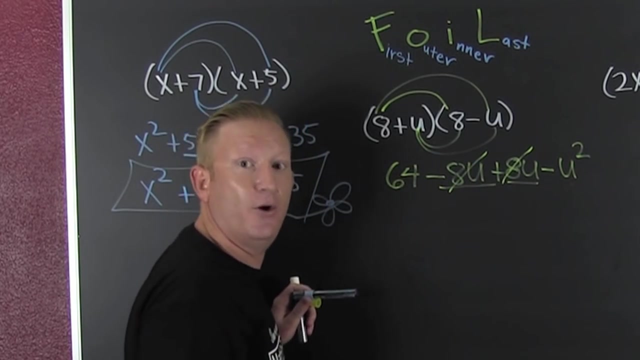 Oh boy, Minus 8u. And then we enter: That's plus 8u. And then we last: That's minus u squared, Because minus times plus is minus u times u is u squared. And then we gather, collect and combine. Oh, We see we have additive inverses. They fight, Oh, They go away. It's special, You're going to find out that it's special, You're special. And then that's special.